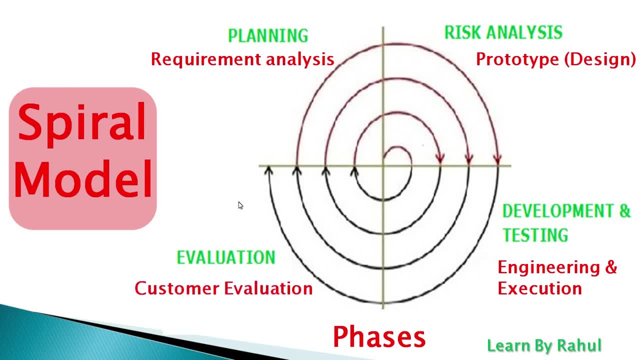 Or customer evaluations. So here we directly give the software to the customer And we take the feedback from the customer To ensure that, as per the requirement, our software is working fine or not. Then again we move on the first part planning. Then again we gather the requirement. 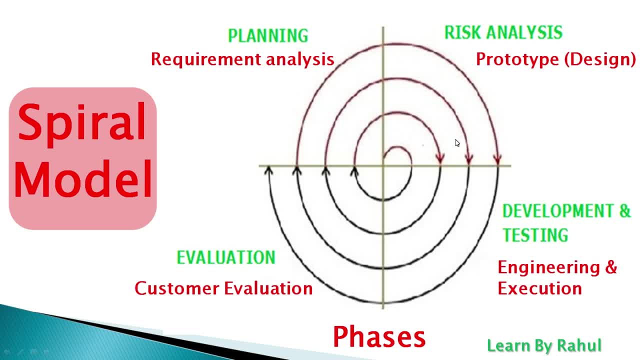 Then again we go for the risk analysis, Then again development and testing, Then again we take the customer evaluation. So we again repeat all phases till customer rate is not satisfied, Okay. So it is also called iterative evaluation. It is also called iterative and incremental model. 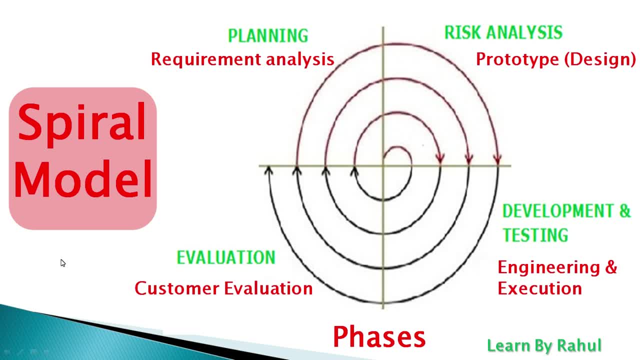 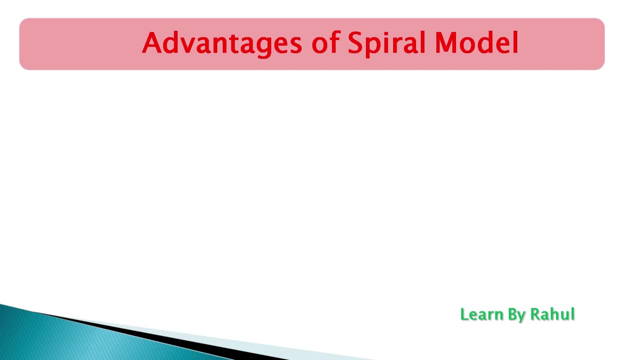 Why? Because we can see. we repeat all phases again and again. We gather requirement, Then development, testing, evaluation. So that's why we call it incremental model as well. So let's move on advantages of SPIRE model. The first is best approach for testing and development for complex and large project. 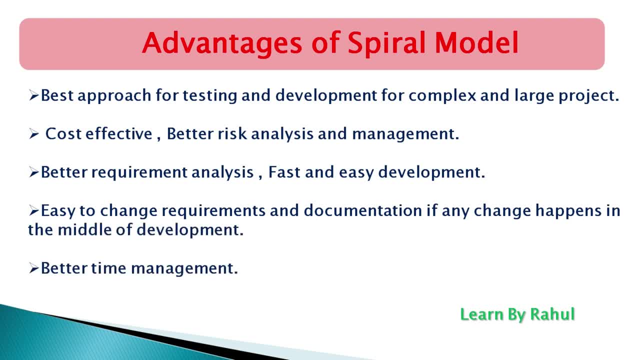 Okay, The second is cost effective: better risk analysis and management. Third, better requirement analysis. fast and easy development. Fourth, easy to change requirement and documentation If any change happens in the middle of the development. And the last, better time management. 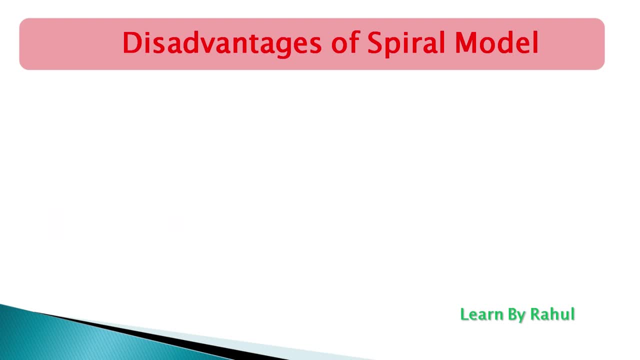 Then we move on the disadvantages of SPIRE model. The first one is difficult to follow, strategy For small project, Not much useful for low risk projects, Need for experience resources as process is bit complex And the last large documentations. So let's we talk about when SPIRE model should be followed. 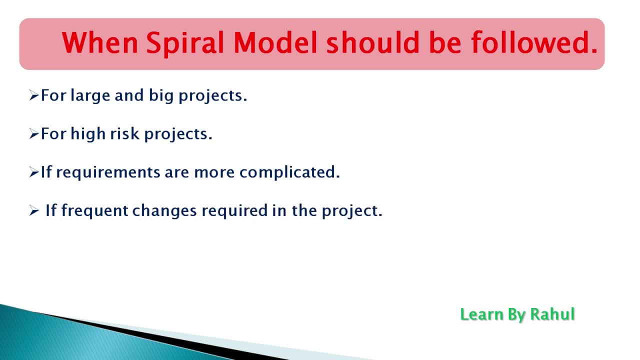 For large and big projects, For high risk projects If requirement are more complicated, And the last, If frequent change required in the project. So this is all about SPIRE model. If you like this video, you can subscribe my channel for more videos. And if you have any query, please comment below. Thank you.